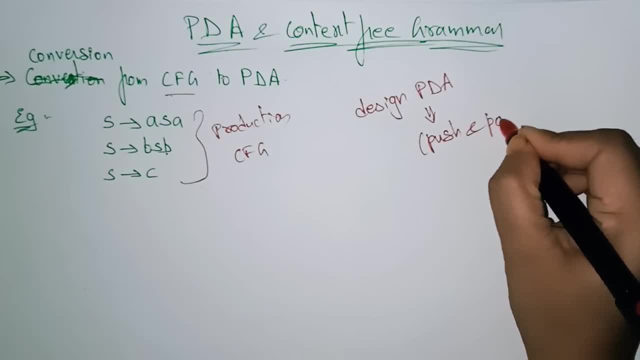 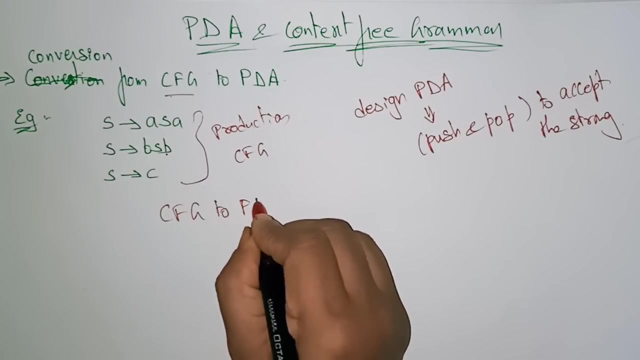 so we have. we will do push and pop to get to accept the string, to accept the string. so this is a method we follow. okay, for context free grammar to push down automata. what we have to do to convert the context free grammar to push down automata. what you have to do: 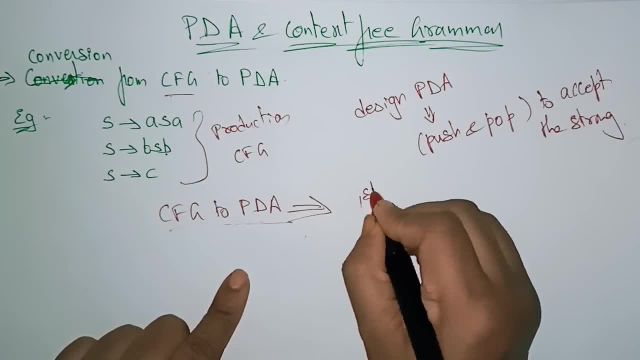 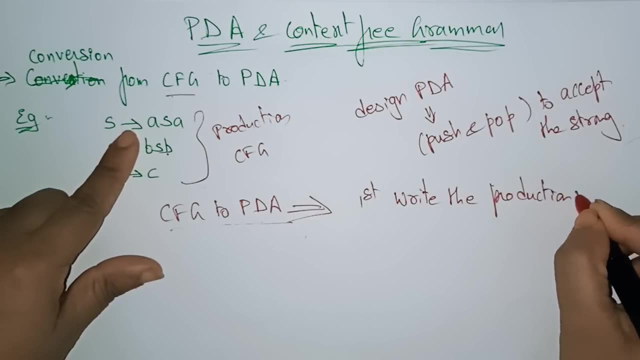 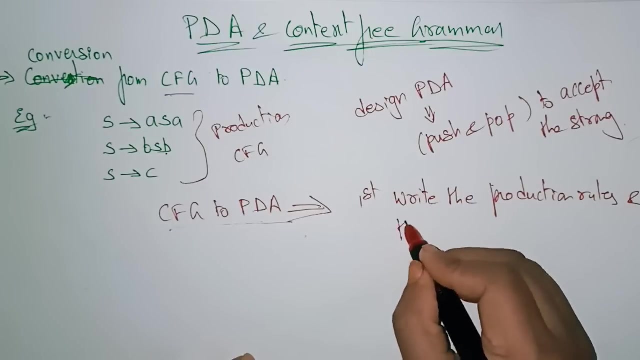 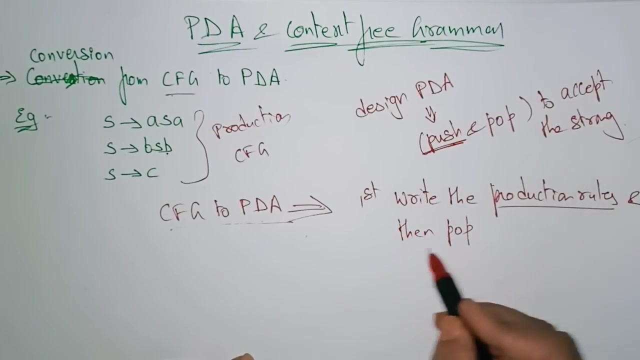 simply first write the productions, first write the production rules. whatever the production rules are there, first you write the production rules and pop and then pop the elements. so here you are not using the concept push, you just write the production rules, after that you pop the elements. okay, so there is no pushing here, only production. 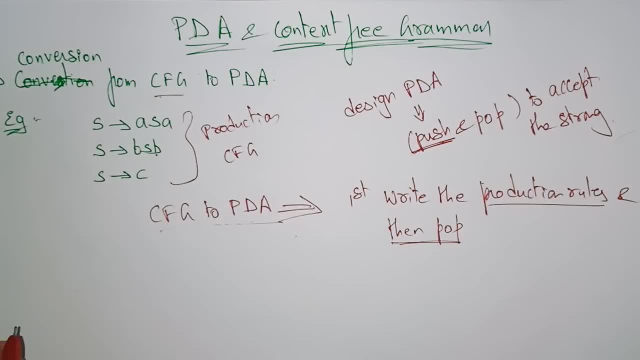 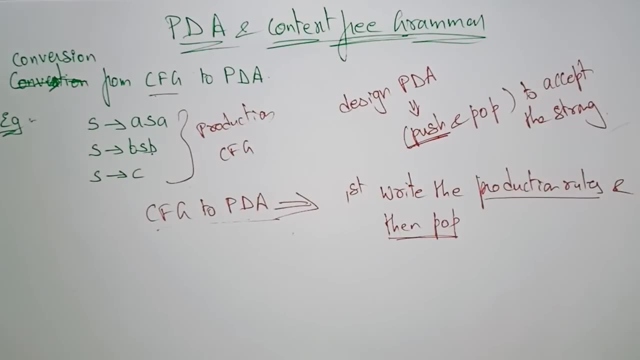 rules and then you're popping that. then you can convert the given context free grammar into push down automata. so let's start the problem. so first starts with the production. so first thing is i have to write all the production rules and then pop: so these are the production rules. that has to be. 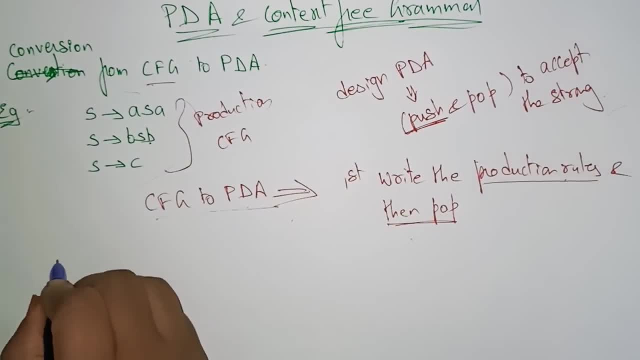 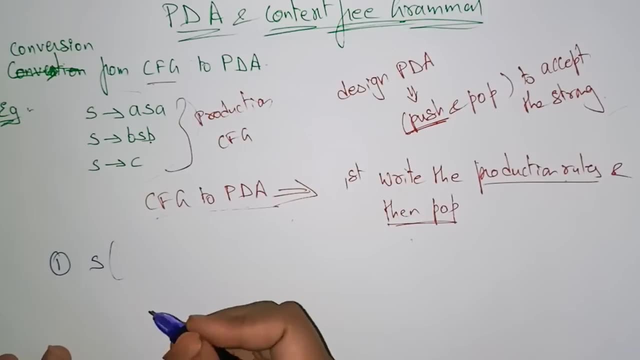 represented in the pushdown automata. so the first one. the first one is: i have taken this s write. the id. id is a instantaneous description, so that you have to be right, instantaneous description is starting state. i am taking as a q naught, q naught, okay. 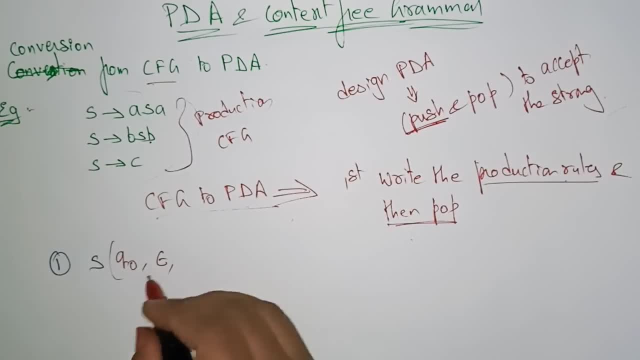 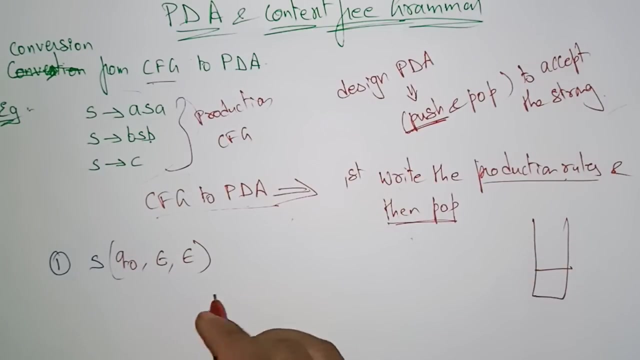 at starting nothing is there. epsilon, that is a start input symbol, is null. okay, that input- i am reading it's a null. okay, there is nothing. is there in the stack? now? the stack is empty. q naught is a start state. the stack is empty. that is a string i. i didn't take any string. uh. this is the uh we are. 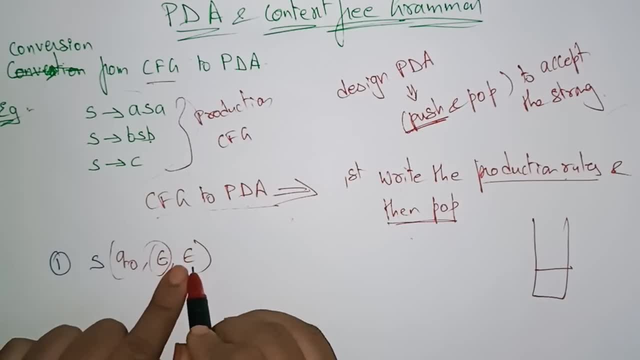 input symbol. we are taking only the null. okay, now the stack top of the stack is epsilon. nothing is there on the top of the stack- epsilon. okay, we are working on. the input symbol is null, because i don't know what are the input symbols. i'm just reading the production. so here there is no for the state. 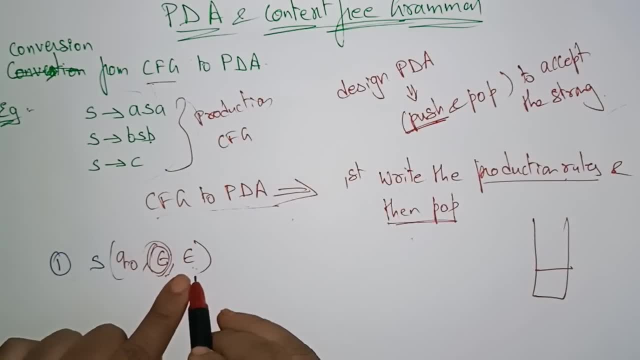 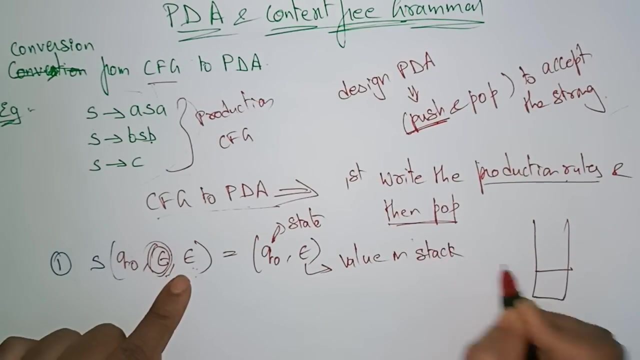 eight, there is no input symbol and the top of the stack is epsilon for this q naught comma epsilon. so here the q naught is nothing but the state. here the epsilon is nothing but the value on the stack. so, starting there is no value on the top of. 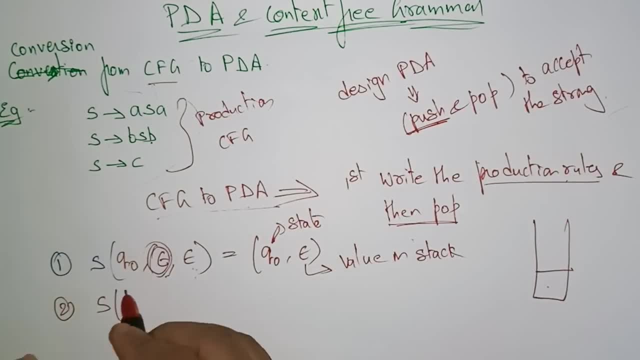 the stack. now, coming to the second stack contains s. is a stack contains q. naught, now, the start input symbol is a null symbol. okay, now i have taken this s top of the stack, top of the stack s i placed on the top of this stack. so what is the top of this stack? write the production rule. what is the top of? 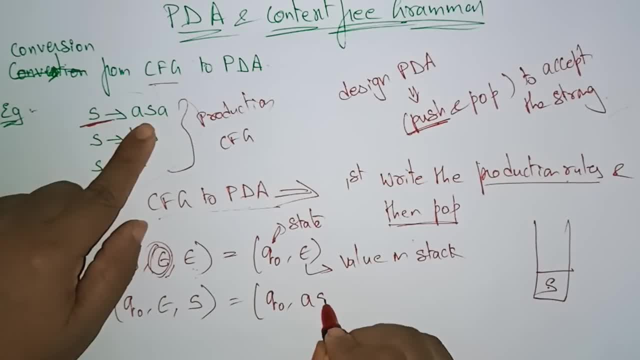 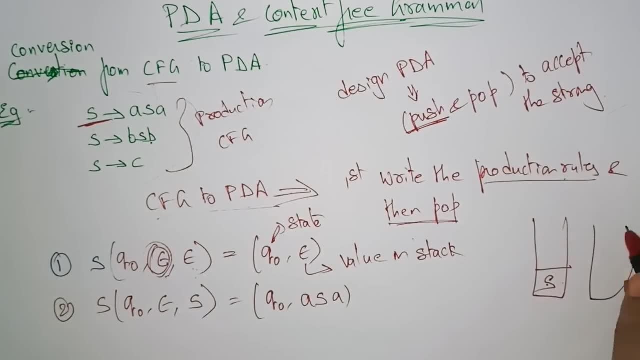 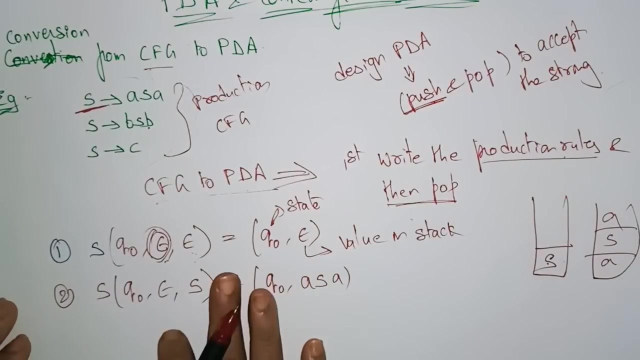 this stack, the top of this stack. that production rule is a s a. so in place of a s a, you have to write a s a. okay, a right, a s a, like this top of this stack. so this is just one production rule means i'm writing only the production rule. i'm not doing, i'm not performing the all operations, i'm not. 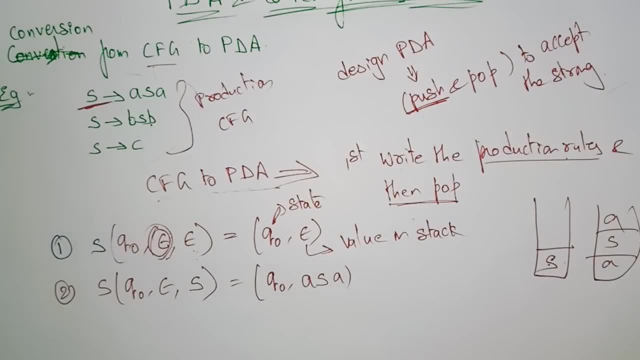 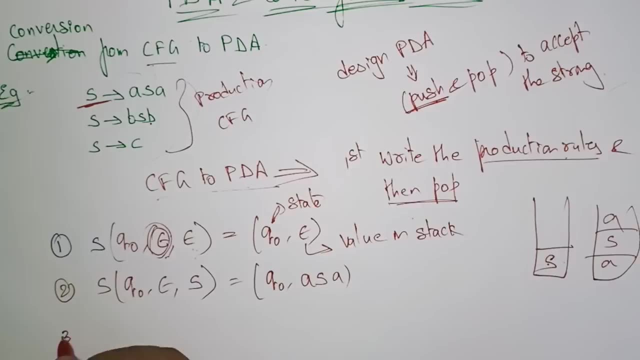 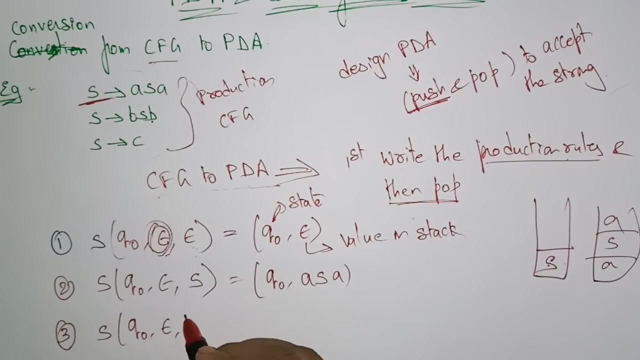 performing. i'm just writing the rules. after that i take the transition table to convert the context free grammar into the pushdown automator by seeing this production rule and i'm not doing production rules next. there you can call the transition rules. next is s q naught epsilon. okay, 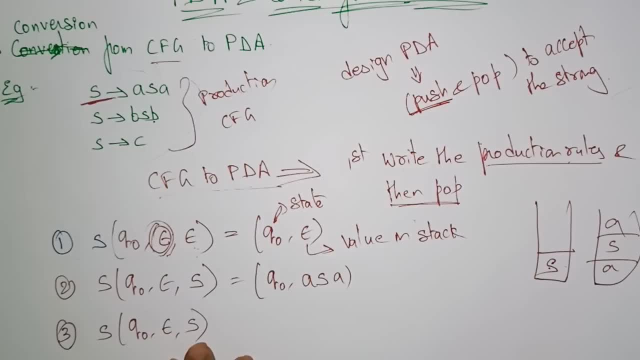 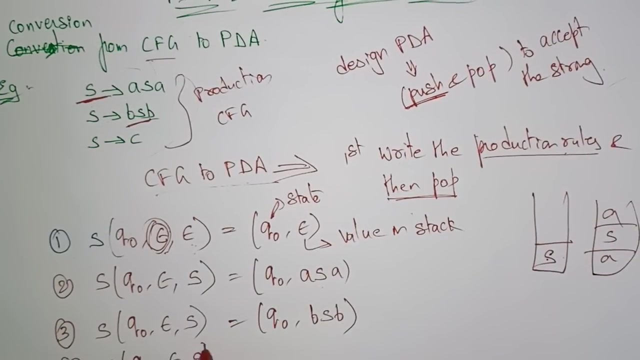 start top of this. uh, that is the start. s is a start symbol s top contains: this is this time, instead of asa, i'm going right- the bsb, bsb. this is one production and the fourth rule: q naught epsilon. the top of this track may be q naught comma c. 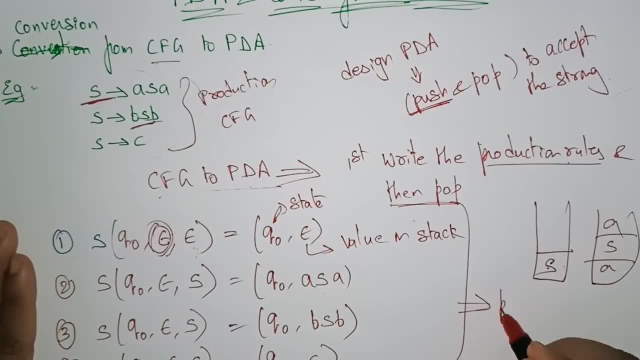 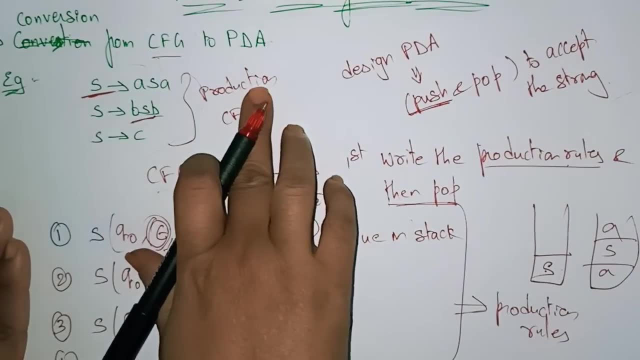 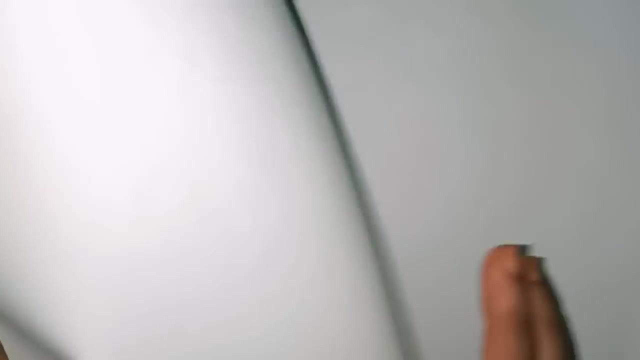 okay, so these are. i have written all the production rules. production rules. so according to the uh method to convert the context free grammar to production rule, first write the production rule and then pop. so i have written all the production rule. now i start the operations of doing pop, the fifth transition. so here popping is taking place. the production rules: there are no. 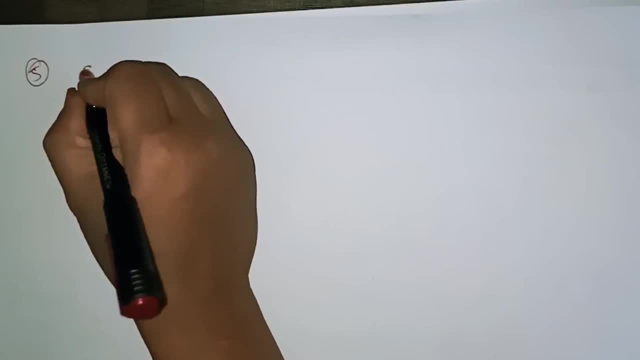 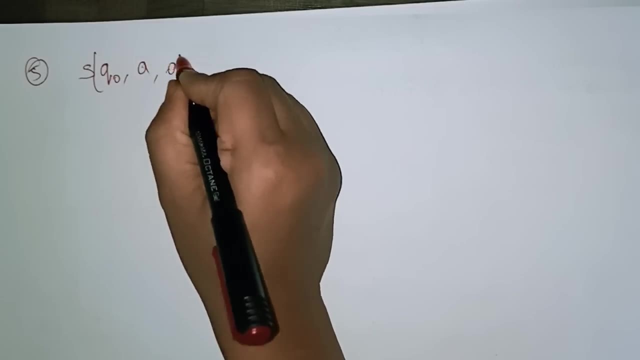 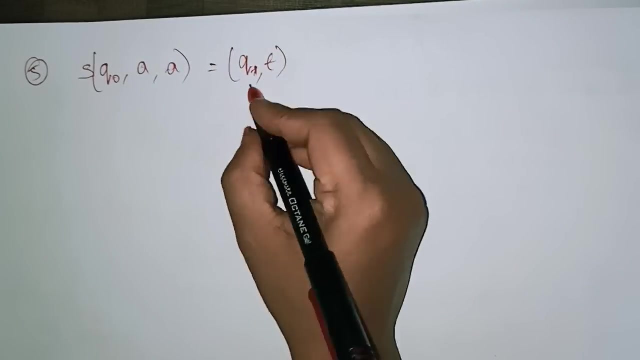 input symbols. now i'm taking the input symbols to pop the stack s, q naught, so there is no input symbol. now i'm placing the input symbol, a, okay, and the stack contains the a, q comma epsilon. so q1 comma epsilon means the changing the state. so whenever the it is changing. 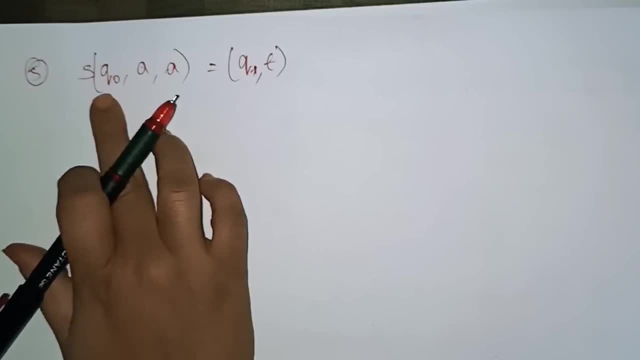 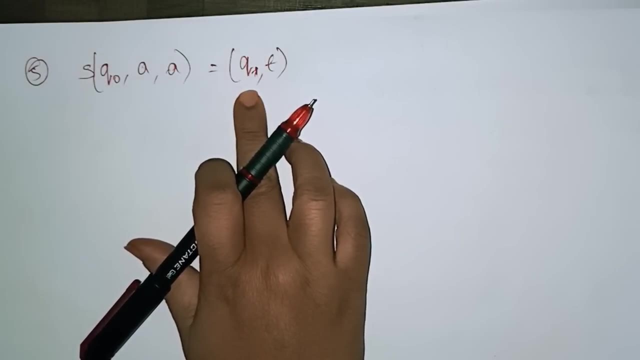 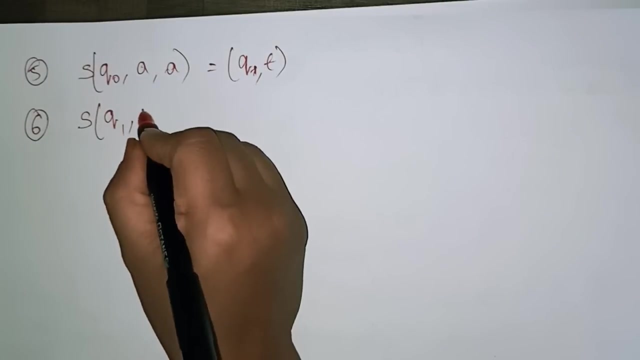 the state, the uh. changing the input symbol means epsilon, means you are entering one state. it changes the state q naught to q1. okay, change of input state has to change the state now. sixth rule: stack contains: now: the new state is Q1.. Next time, placing the input symbol B: Now the top of the stack contains the B. 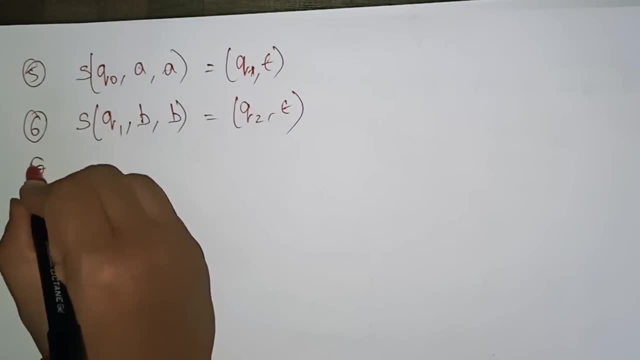 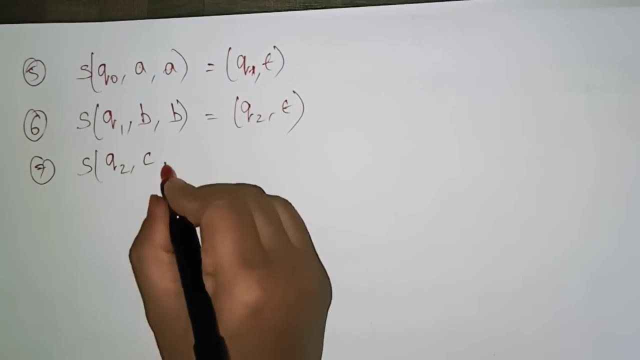 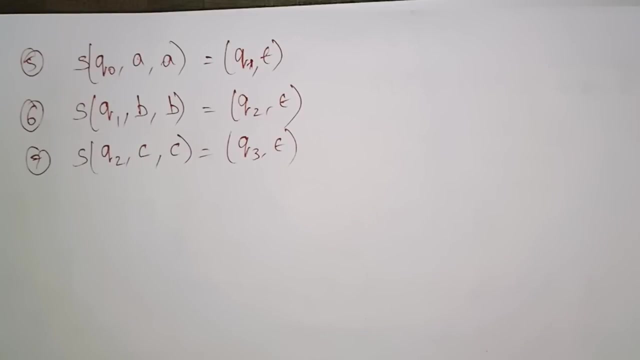 It changes the state to Q2.. Now the 7th transition: S. It changes state Q2.. Now the top of this. now I am placing the input symbol C. Now the top of this stack is C. It changes state to Q3, comma, epsilon. So these are all the rules. Now take the transition table. 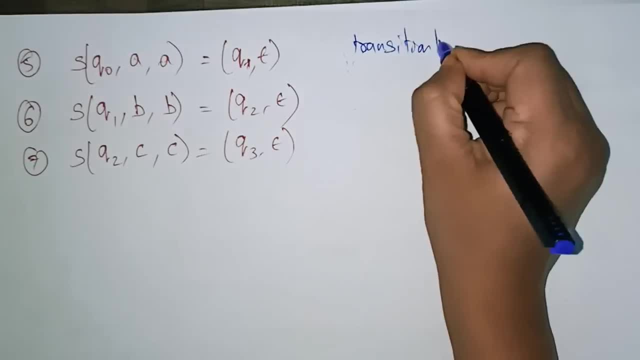 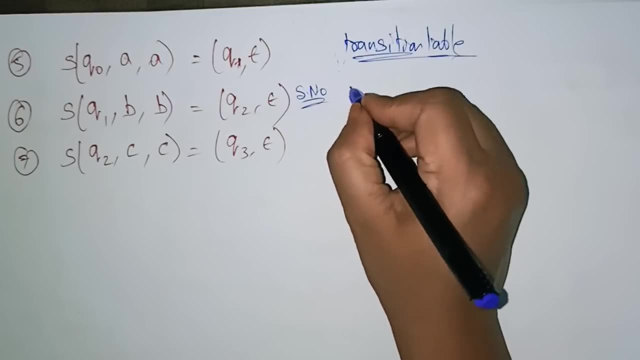 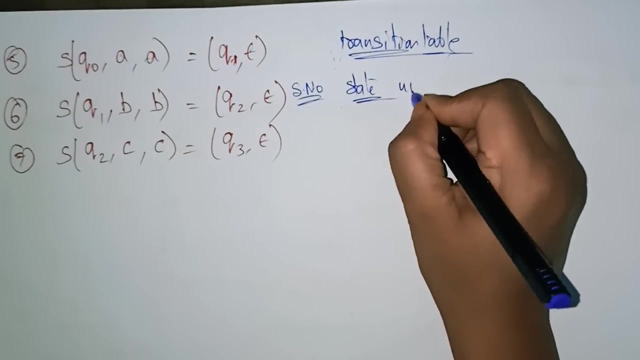 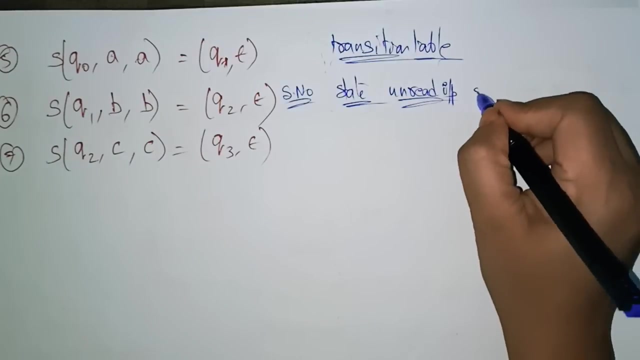 Let me write the transition table. Okay, So let's take the serial number and stack state, whatever the state that it contains at present, in which state? and unread input, that is, a unconsumed input. that is there in this unread input and what is there in the stack? Okay, And the transition number, which? 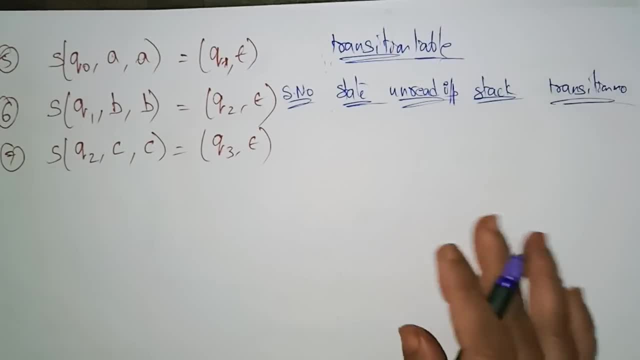 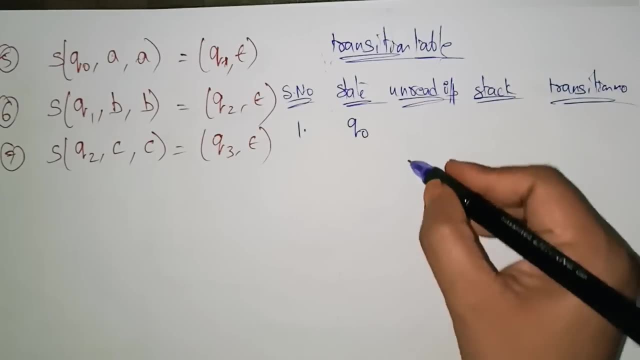 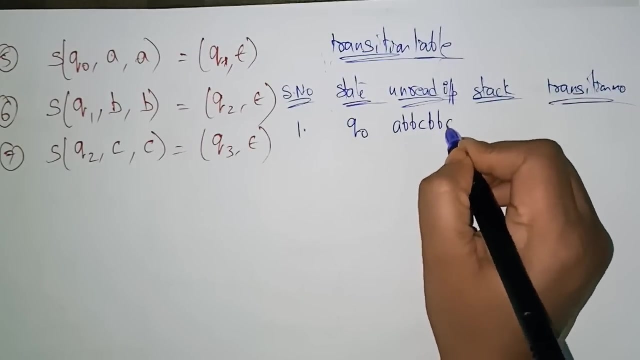 translates number is applying on that that. you have to be right. transition number now start. so starting the state should be q naught. this is the initial state. let's take a string, unread input string. whatever the string you want you can take, but here i am taking a, b, b c, b b a. this is a unread. 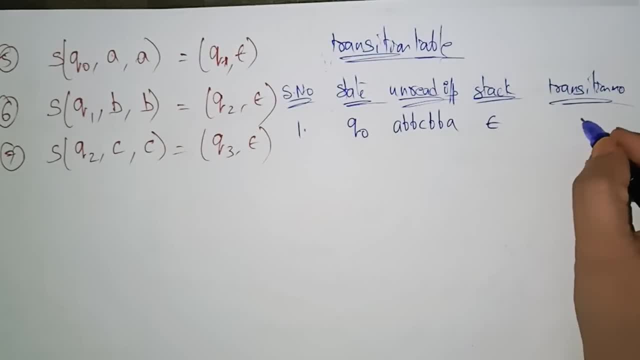 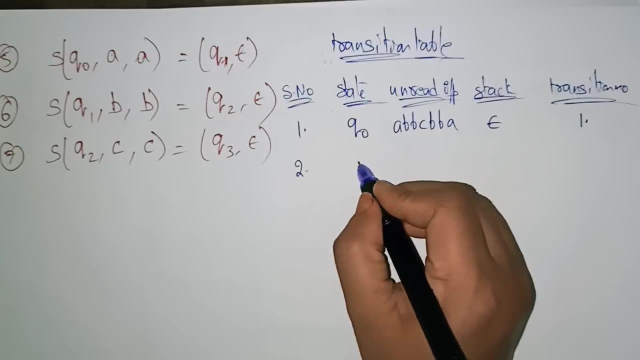 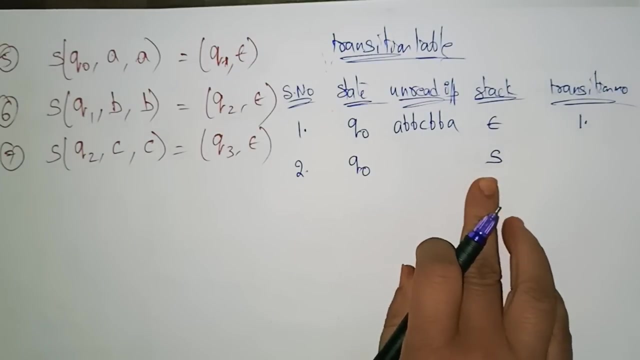 input string i am taking. initially, the stack is empty. this is the transition one. okay, the first rule i am applying. second, okay, second is state: is q naught, q naught, i in the stack i am placing the top of the stack is a start symbol. okay, this is a s is a start symbol. the unread input data is: 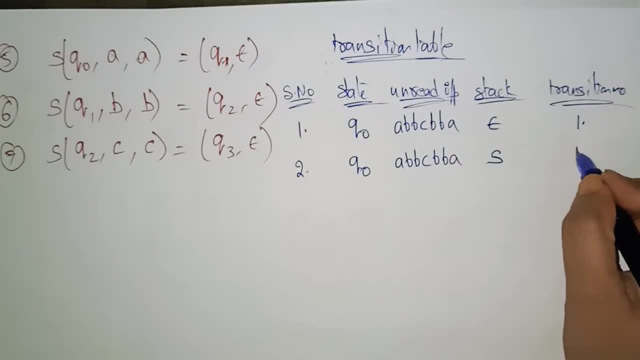 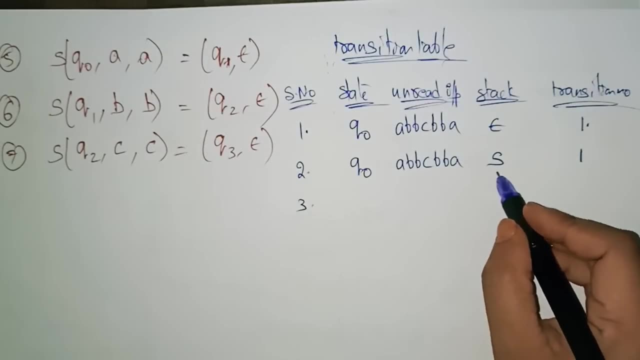 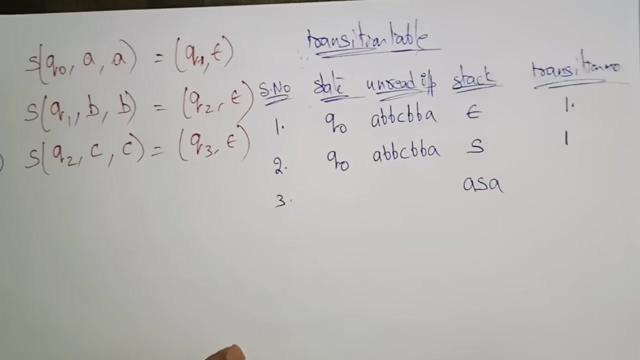 a, b, c, b, b a. so i use the transition number one. okay, because that is a transition three. now, in place of s, i am placing the top of the stack as a s a. so which production i have used? which production i used here? a s a, a s a is a second transition. 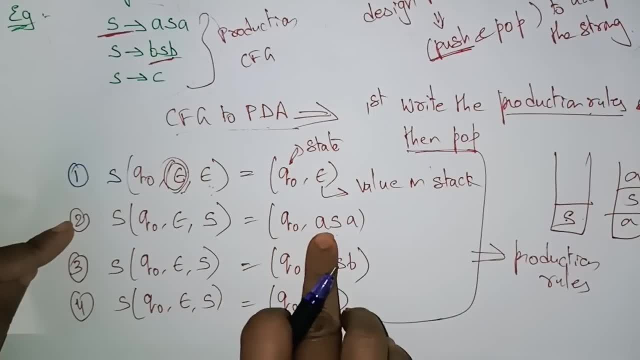 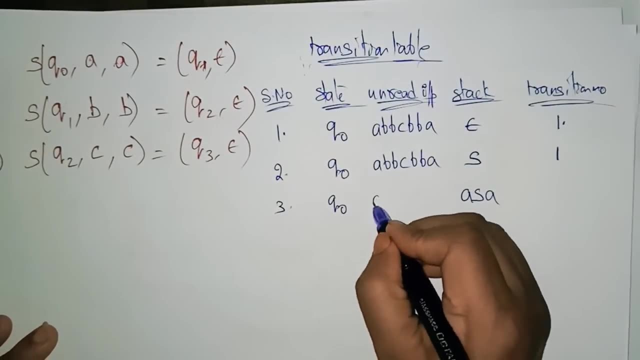 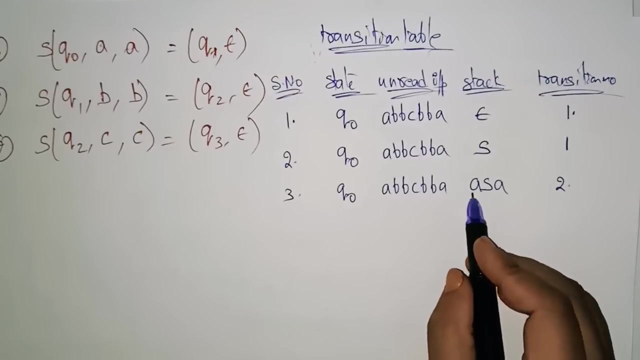 so here the state is similar. q naught is only in place of s. i place a, s a. the state is q naught. only the input is a, b, b c, b b a. i had used in the transition state as two. now check here the stack. 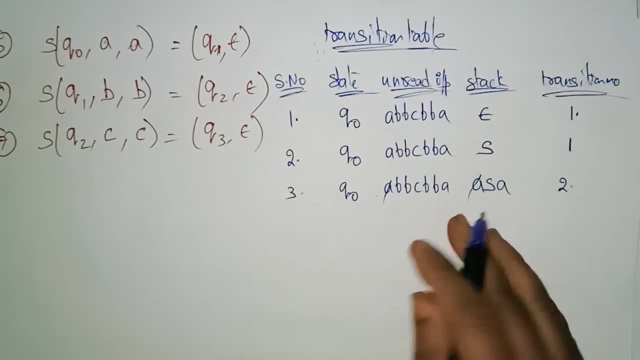 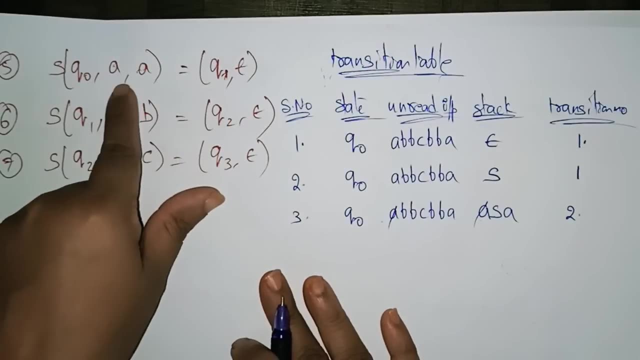 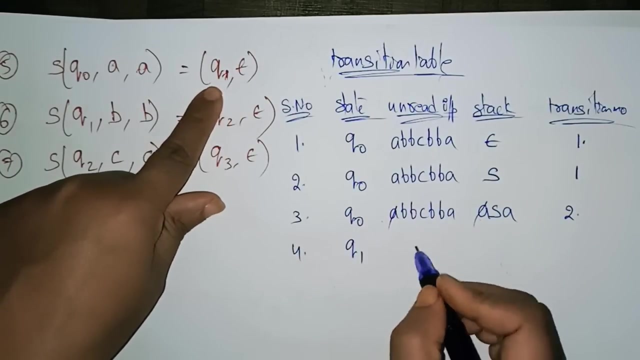 contains a and the unread input data. is this similarly similar? so pop it. so popping. popping means whenever we are popping, the state is changing here. okay, if a is there, i need to pop. epsilon represents the pop. okay, so now the state changes to q1. now the stack, uh, unread data is b, b, c, b, b, a. now in place of years, just write s, a here. 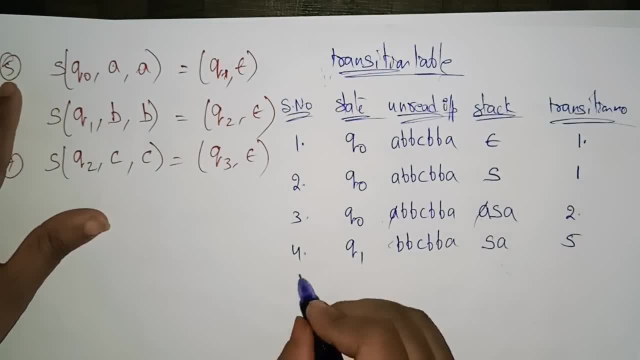 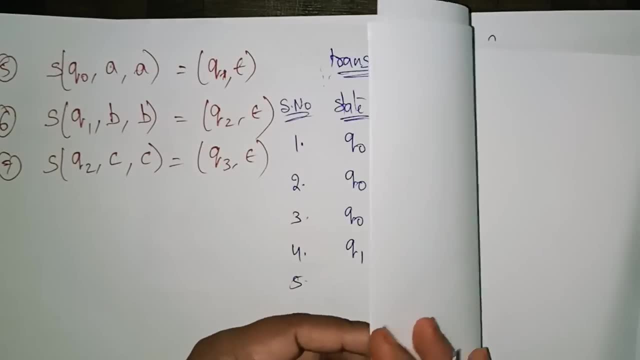 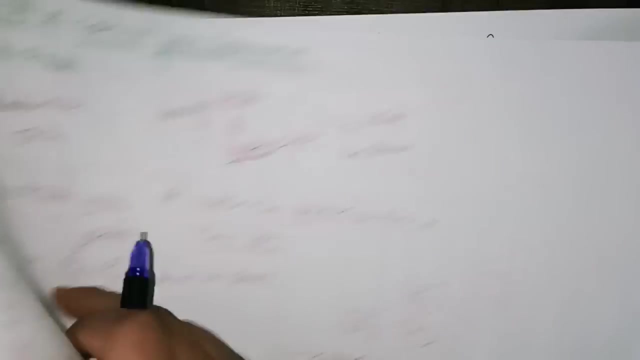 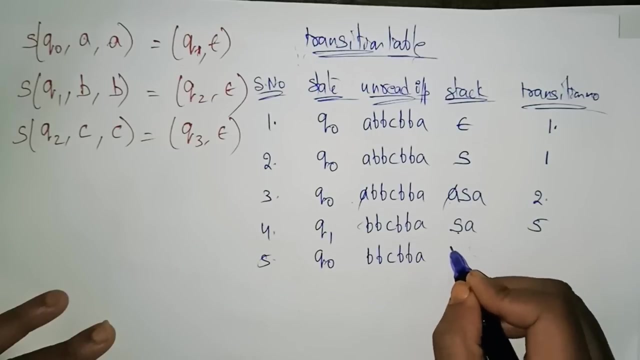 so i have used in the transition number rule five, now fifth. so here in place of years i am writing this time b s b. so which rule it is? b s b, b s b is a third transition is a state changes. no state changes to q naught. so now the state is new state is q naught. b, b, c, b b, a. now s is replaced. 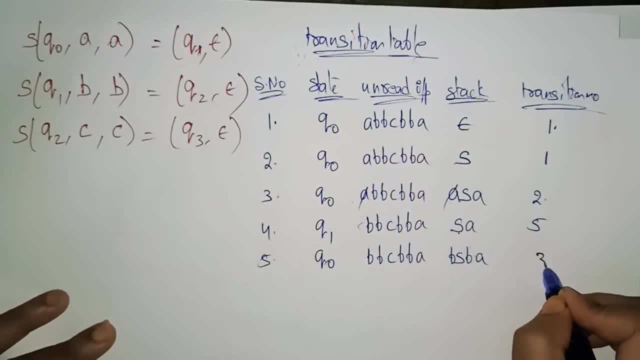 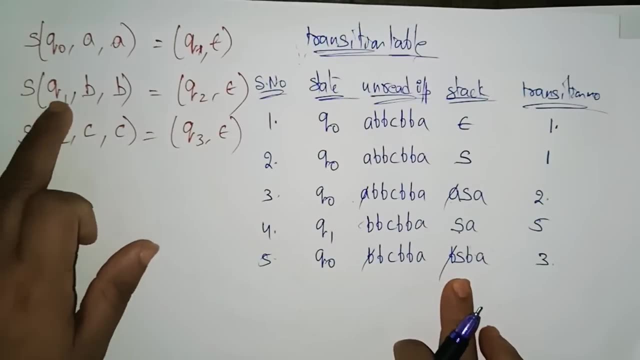 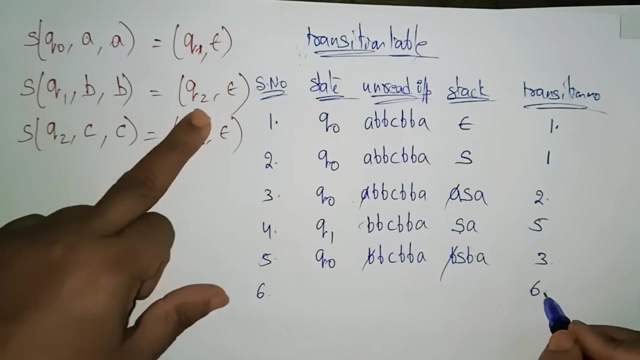 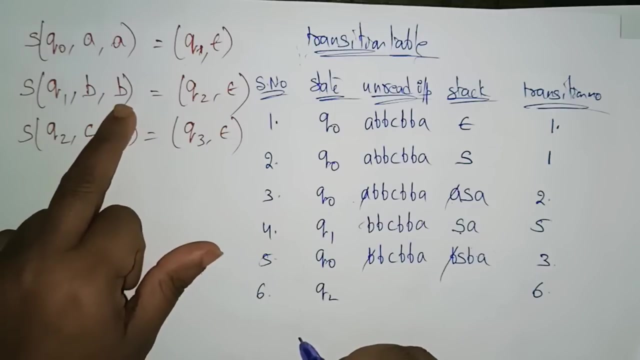 with b s, b a, we are using the third transition, third rule, so same elements are there. b then pop it. so by seeing the rule which rule sixth. okay, so this is a transition number six we are using to pop now the state changes to q2. so because for input value b you need to the top of the stack b. 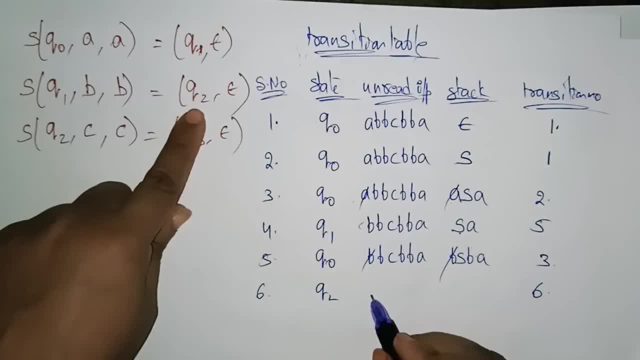 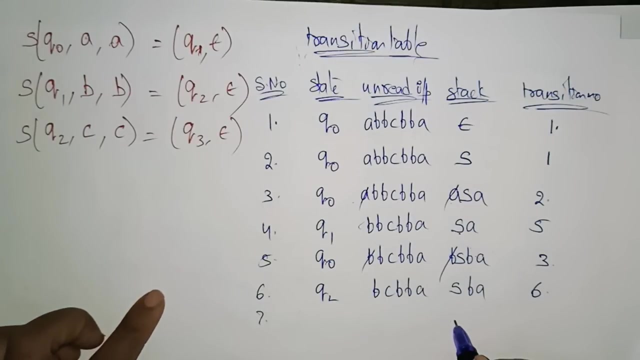 you need to pop it, so i popped it. the state is changes to q2 b, c, b, b, a now. this is s b, a now. in place of yes, i am writing c b a. okay, in place of yes, i am writing: let me write here one more b is there now, so again write. 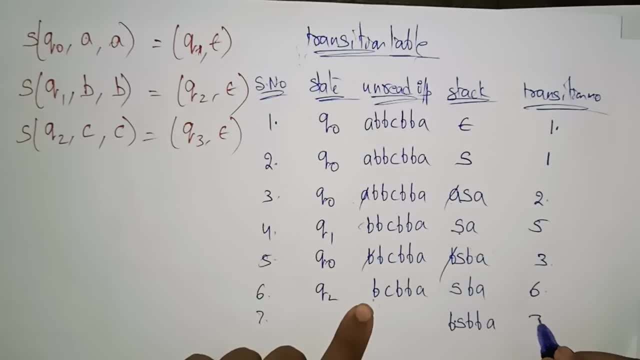 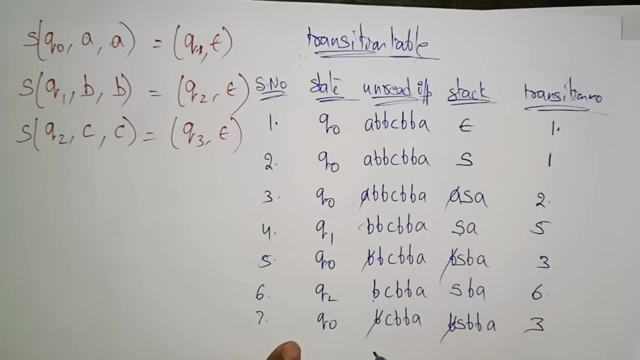 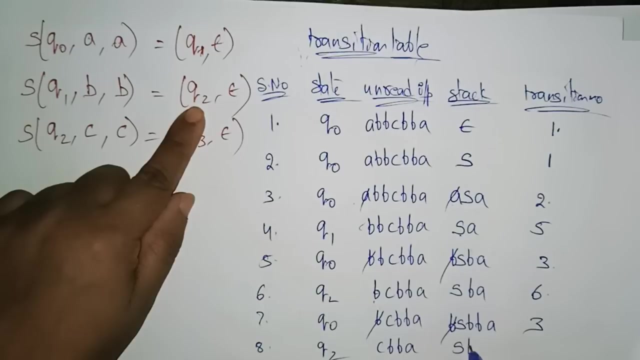 b, s, b, b a. so according to the rule three now the state here is the q naught b, c, b, b, a. so here the same elements are there, so pop it. pop it means the state is q2 c, b, b, a, s, b, b a. so i, using the 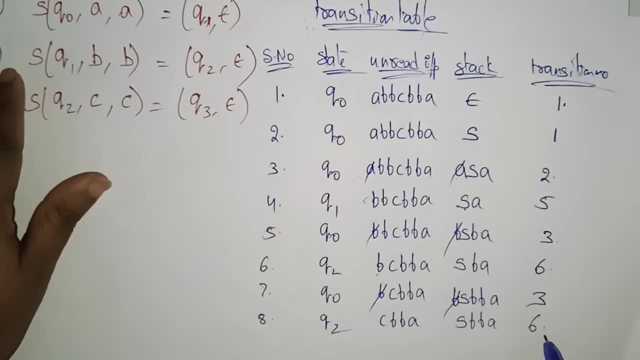 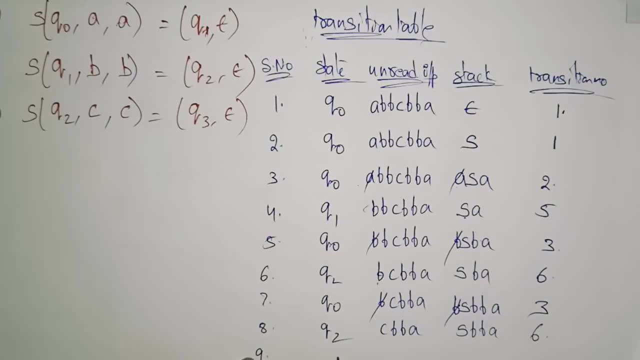 transition state six. i have chosen okay, so sorry, i have popped it now coming to the ninth state. so here c is there. so c means in place of: yes, i can replace s with the third production, so this is a three i can afford. i can replace in place of: 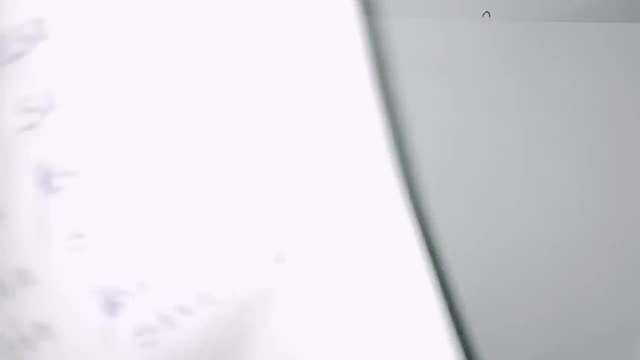 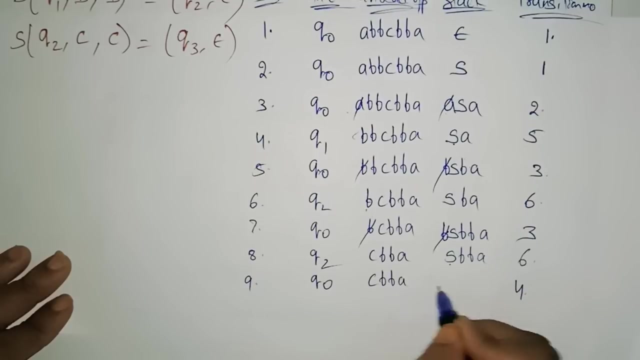 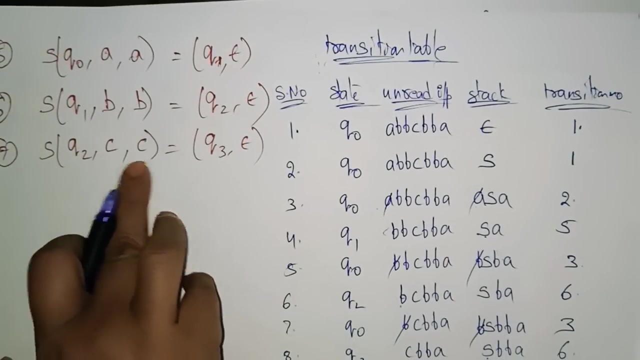 yes, i can replace with the c, so that is the state. is q naught? that is, i have using the four four transition state. is the q naught? c, b, b, a in place of yes, i am writing b, b, c, b, so pop it so by using the production rule seven. so if 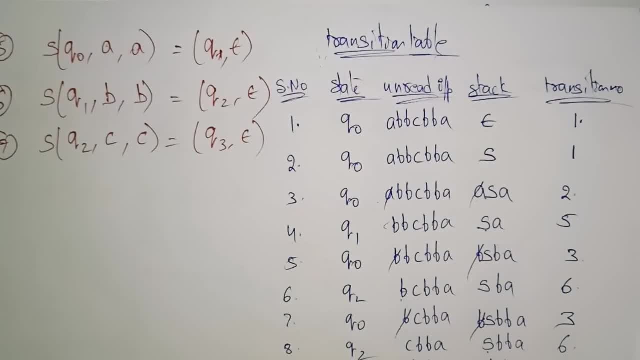 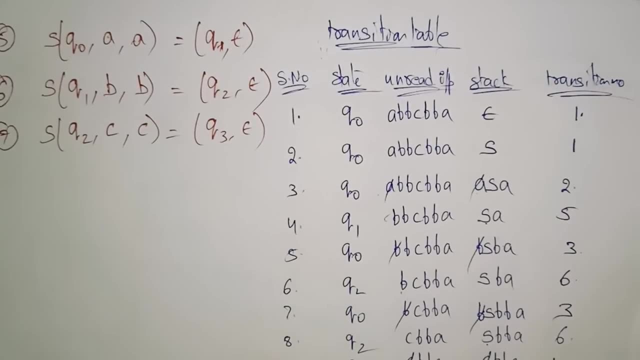 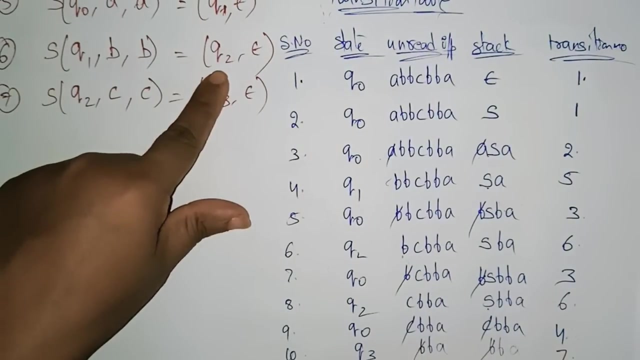 both are same. c means the state is changing to q3, q3, this time b b a, b b a. so this time try to pop all elements, okay, using seven. so b b is there, b b means the state is q2, b a, b a. i have using the 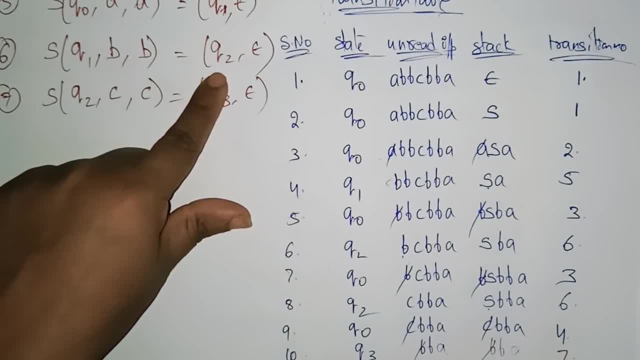 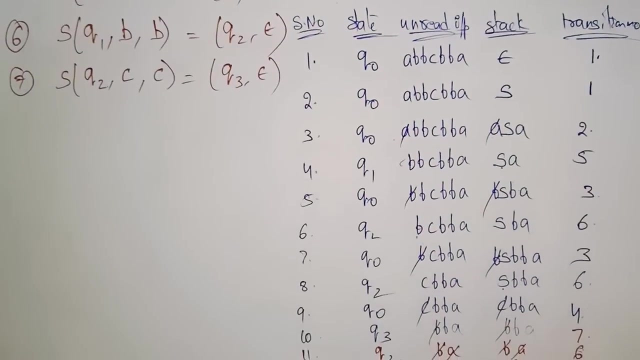 transition c, b, b, a. so this time b b is there. b b means the state is q2, b a, b a. i have using the six twelve, so this time b, b, a will be cancelled again. finally, you reach q1. epsilon a is also cancelled. epsilon reach the final state. so this is how you have to construct the pd conversion. 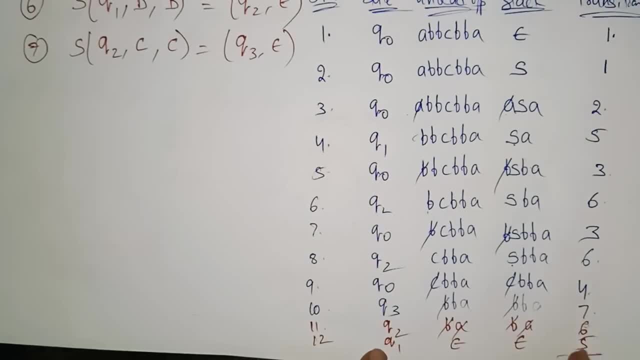 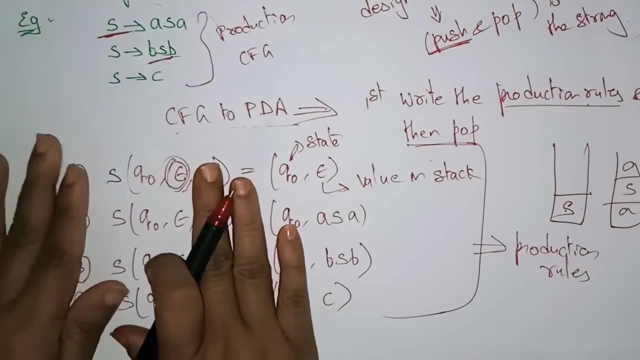 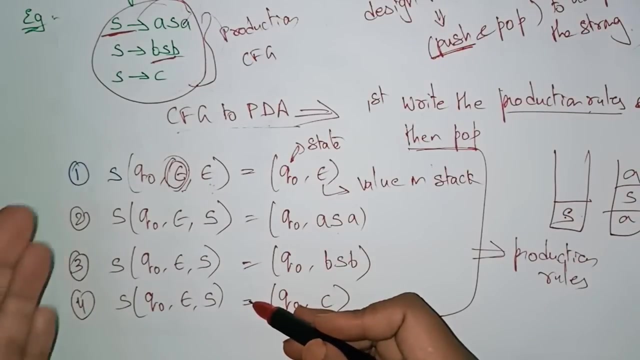 of context free grammar to the pushdown autopilot, i reach the final state. so whenever you reach the final state by using the production rules of pd. so this is, this is a week first here i converted the context free grammar into this pda. these are all the pda. the problem pda is this: production rules- okay, pushdown automata. production rules. 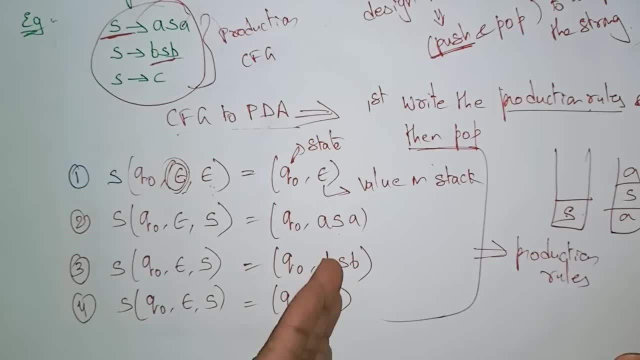 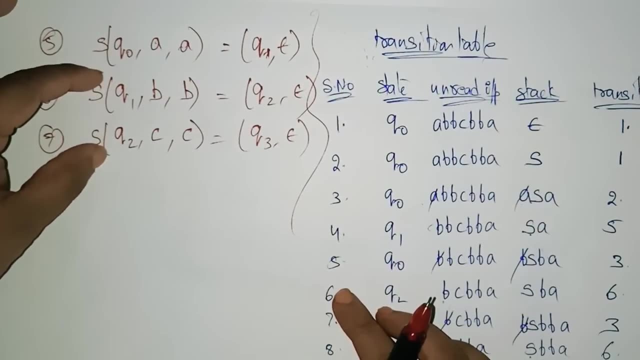 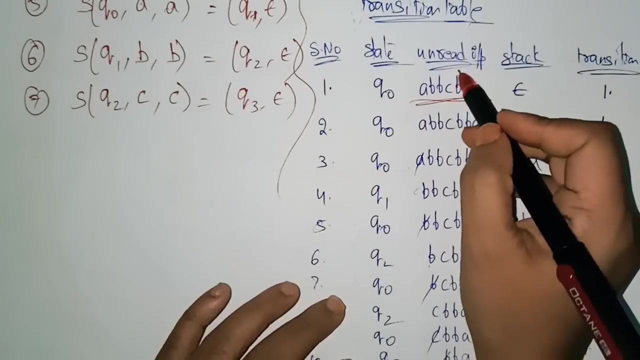 i converted. okay, so first write the production rules and then pop. that becomes the pda. so this part, along with this part, you call it as a pda pushdown automata, uh, transitions. so with the help of these transitions i i taken one input string and perform, and i had pruned. 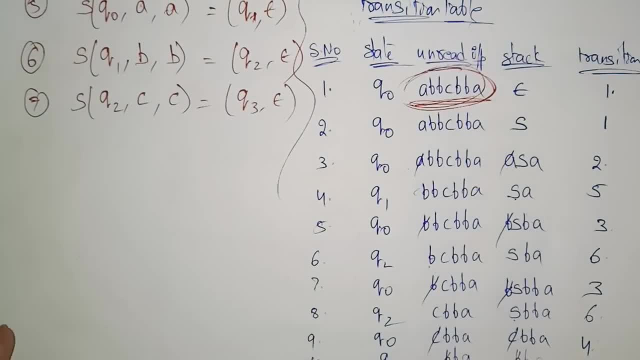 that that, uh, the given, whatever the string i have taken, is accepted by applying these rules. thank you.